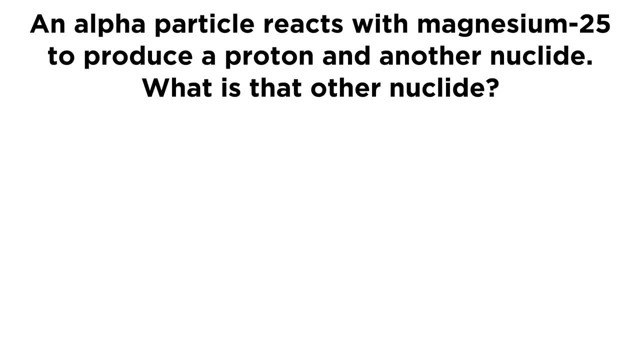 Okay, so let's write out the reaction that is represented here. We know that we are dealing with magnesium 25, so we're going to start with Mg, and that has an atomic number of 12, as any magnesium atom will, and so we put a 12 down. 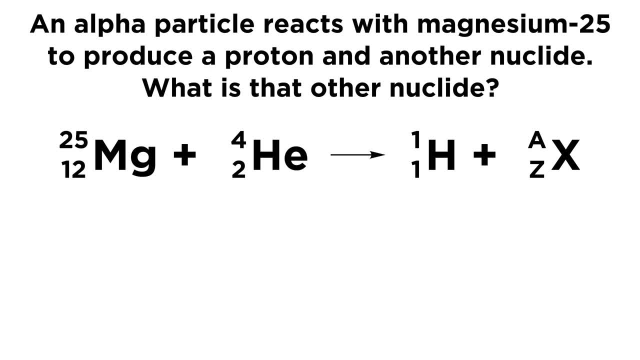 And then this particular nuclide has a mass number of 25, so we can put 25 on the top left. Now we know that that is going to react with an alpha particle. So what is an alpha particle? We have to know that an alpha particle is a helium nucleus, So we can write helium, we can write He. 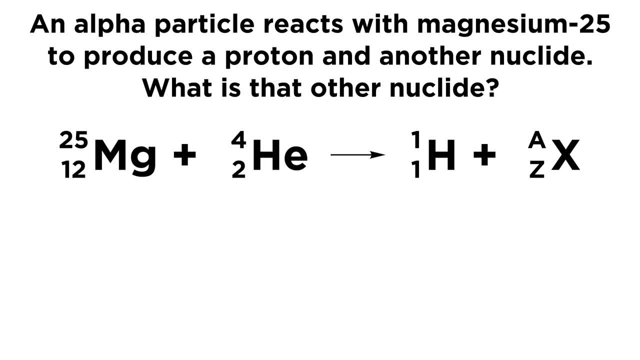 and we know that any helium nucleus is going to have two protons, so we need a two there. and then, specifically, an alpha particle is two protons and two neutrons, so that will have a mass number of four. so we can put a four on the top left. 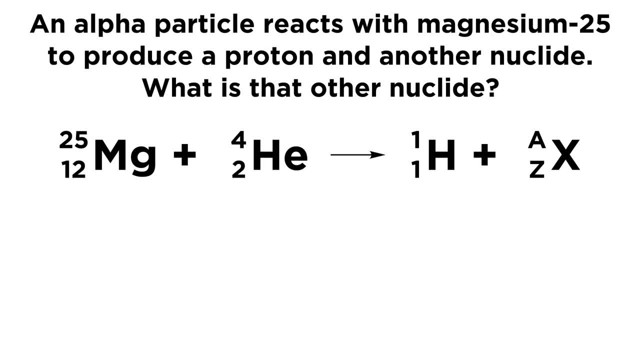 Now we said that we are going to produce a proton. and what is a proton? but a hydrogen nucleus. We know that every hydrogen atom will have one proton in its nucleus. so we can write H for hydrogen, and since there is one proton in the nucleus, that's an atomic number of one. we're going to 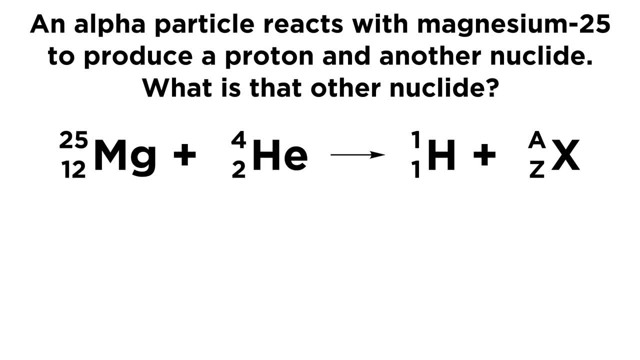 put a one on the bottom left, and since it's just one proton, it's just one atomic mass unit, so we can put a one on the top left as well. and then, lastly, we have another nuclide, We don't know what. 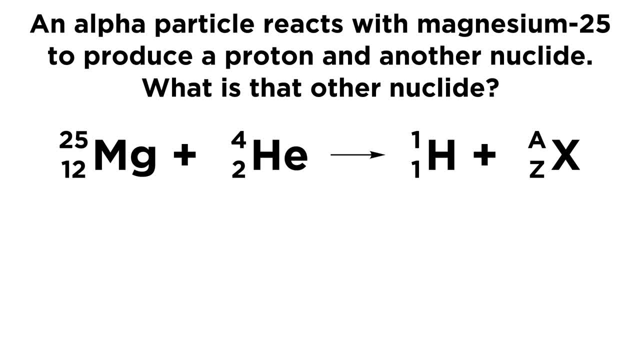 the nuclide is yet, so we can just represent that as x, and we don't know either of these values. so let's just put z and a and we're going to calculate those now. So the atomic numbers and the mass numbers must be balanced. That means that the sum of the atomic numbers on the left side 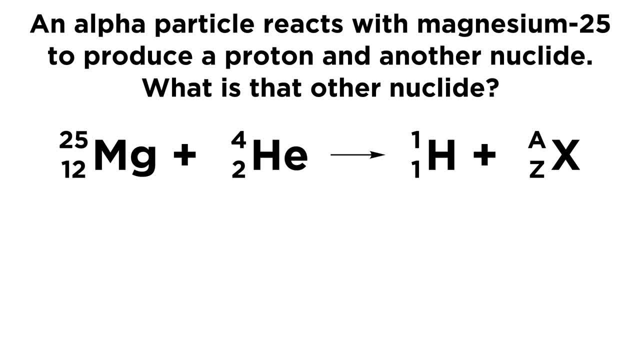 must equal the sum of the atomic numbers on the right side, and the sum of the mass numbers on the left side must equal the sum of the atomic numbers on the right side. So we can put a one on the bottom left here and we're going to put a one on the top right side, and that means that the